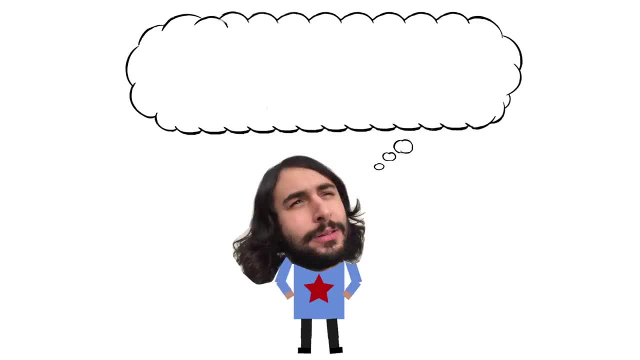 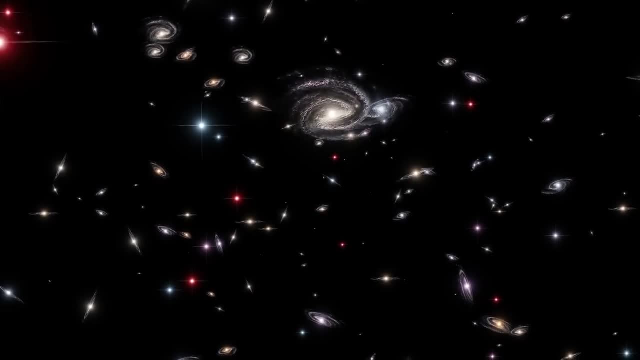 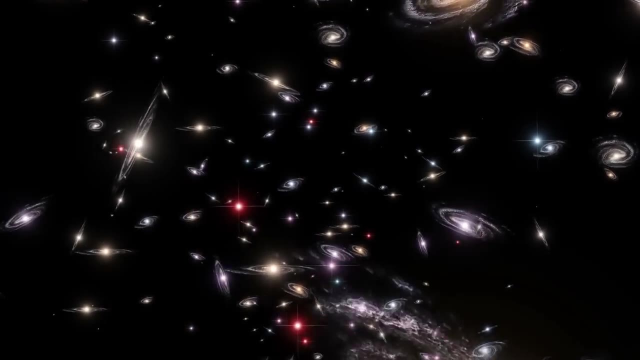 Professor Dave, here let's talk about the Milky Way. We've learned about how stars and galaxies form, and there are hundreds of billions of galaxies in the observable universe, each with many millions or billions of individual stars. So which galaxy is our home? 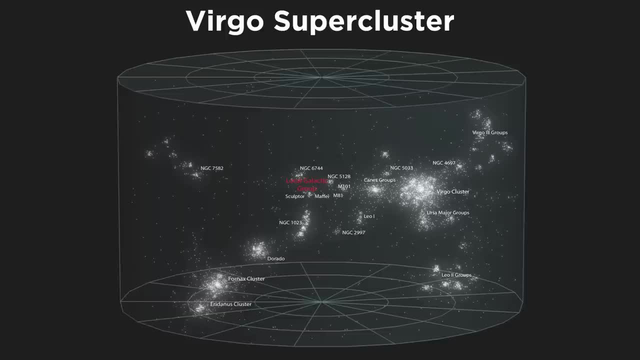 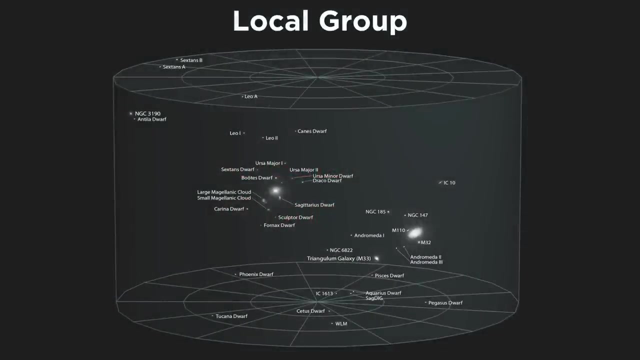 Let's take a look at this collection of galaxies- This is called the Virgo supercluster, containing over a hundred smaller groups and clusters of galaxies, such as the Virgo cluster and the Local Group. Now let's zoom in on the Local Group. 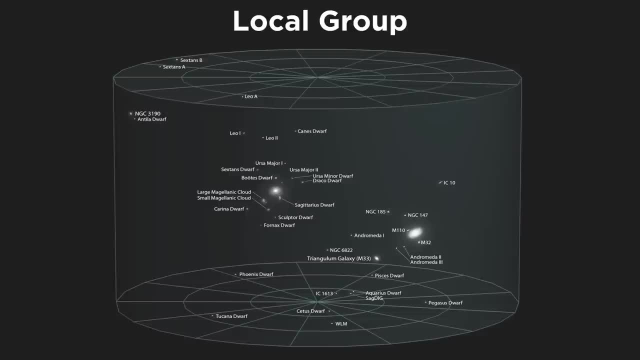 This contains more than fifty galaxies, many of which are tiny dwarf galaxies, but some of which are fairly large by galactic standards. The largest of these is called the Andromeda galaxy, which is a spiral galaxy Around half that size. the next biggest is called the Milky Way galaxy, also a spiral. 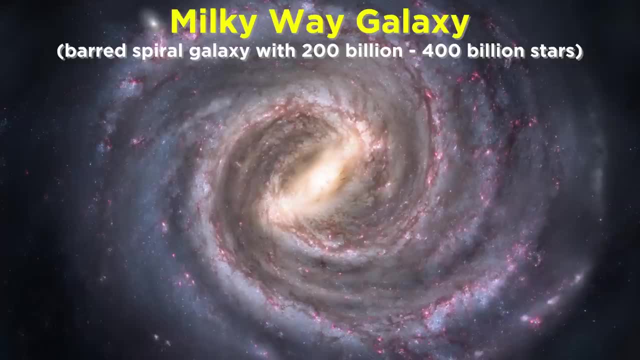 galaxy and that's our home. It's a pretty typical barred spiral galaxy containing somewhere between two hundred billion and four hundred billion stars. It is about one hundred thousand light years in diameter, meaning it takes light a hundred thousand years to travel from one edge to the other, whereas it is only about one thousand. 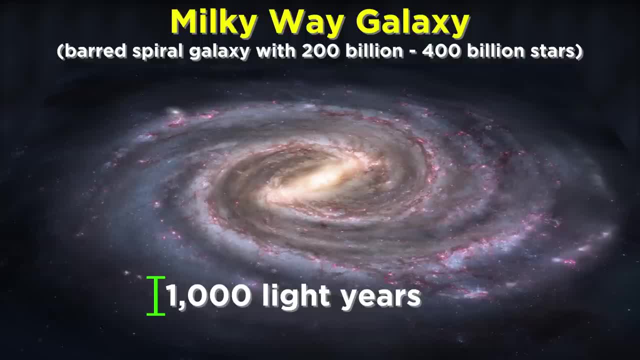 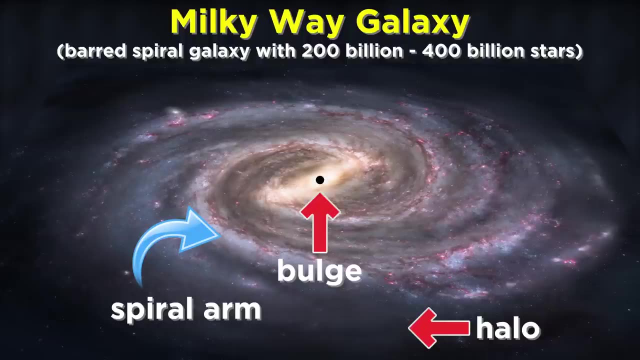 light years thick. These are estimates, as there are no well-defined edges to the galaxy. It is simply a disk with several arms of varying sizes surrounded by a halo of stars, with a dense bulge in the middle, most likely harboring a supermassive black hole at the center of. 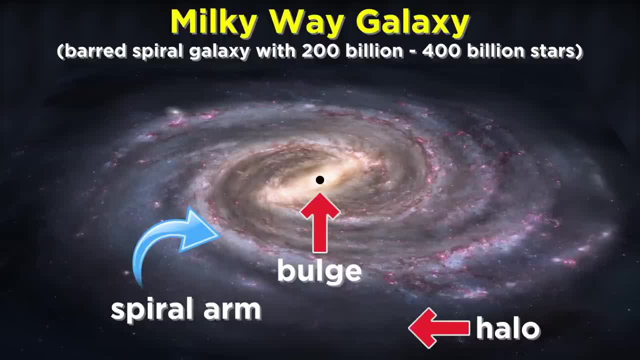 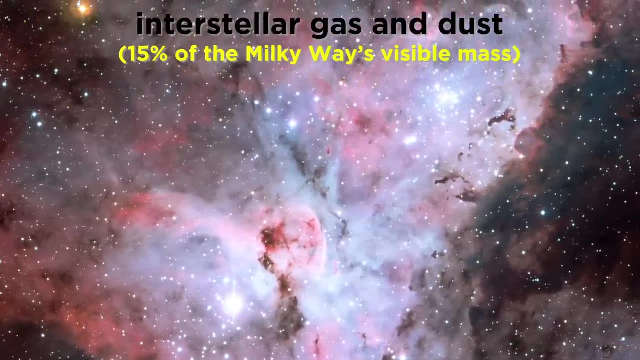 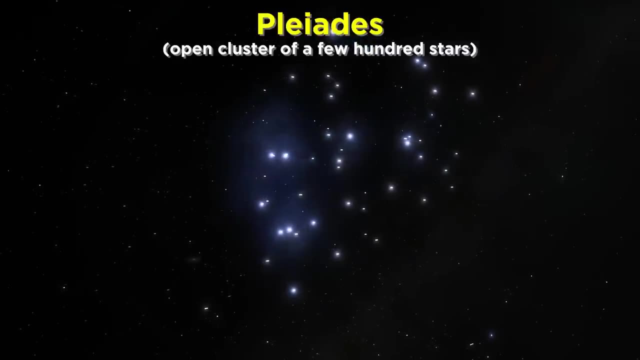 its nucleus, just like other large galaxies. About fifteen percent of the visible mass of the Milky Way is in the form of interstellar gas and dust scattered between all the stars. It's a very large galaxy. Some of these stars form groupings called open clusters, such as the Pleiades, which 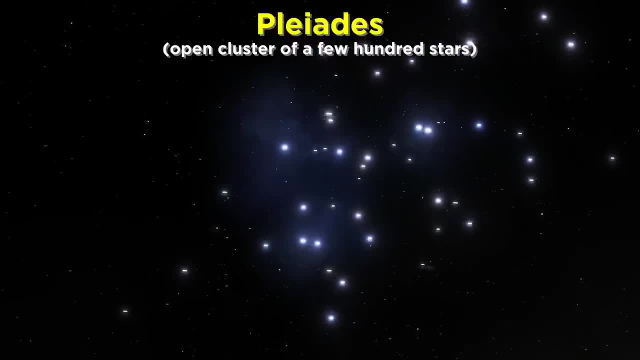 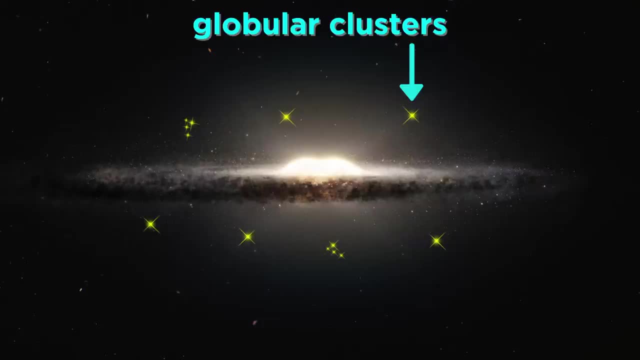 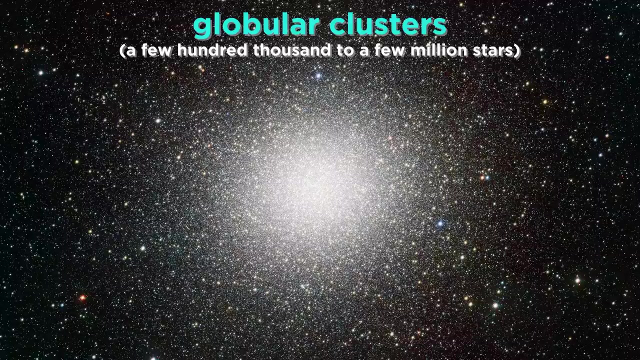 is a few hundred stars bound fairly close together. Beyond the stars in the disk, there are also several objects in more distant orbits called globular clusters. These are dense spherical collections of stars, anywhere from a few hundred thousand to a few million, and there are a little more than a hundred and fifty of them traveling around. 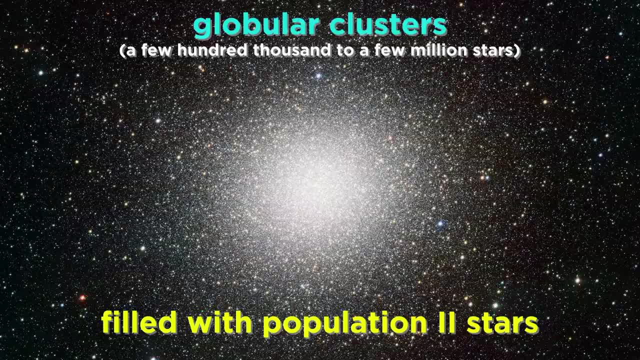 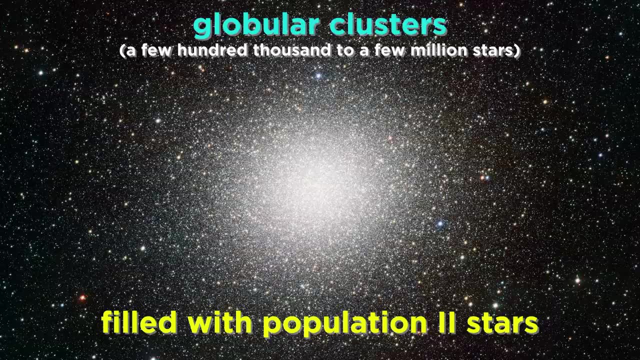 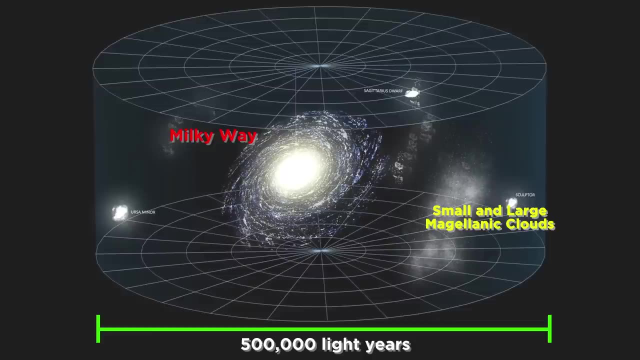 the halo. These are always filled with population- two stars indicating that they are very old, probably forming at the same time as the Milky Way. The Milky Way also has some satellite galaxies, which are smaller galaxies that orbit around it. The most prominent of these are the Small Magellanic Cloud and Large Magellanic Cloud. 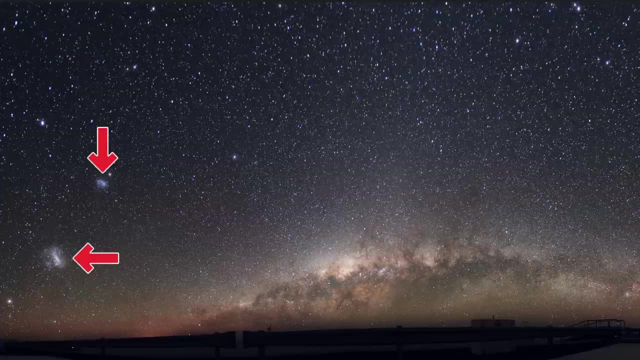 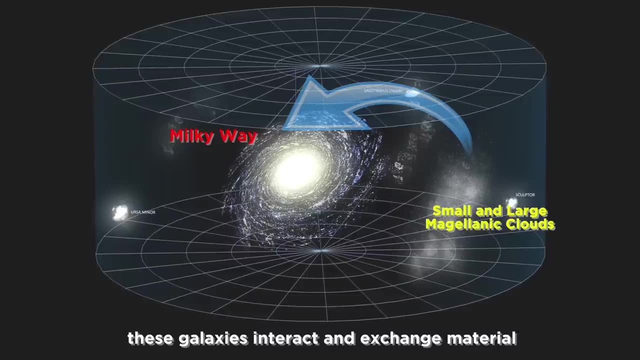 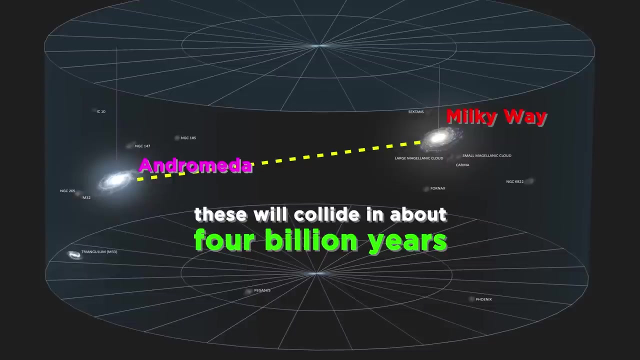 each around a tenth the size of the Milky Way and observable from the southern hemisphere. These interact with the Milky Way as they orbit, resulting in disturbances and also exchange of material. Andromeda and the Milky Way are also on paths that will cause them to collide sometime. 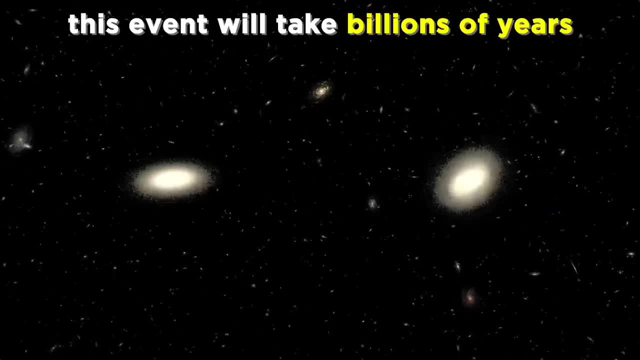 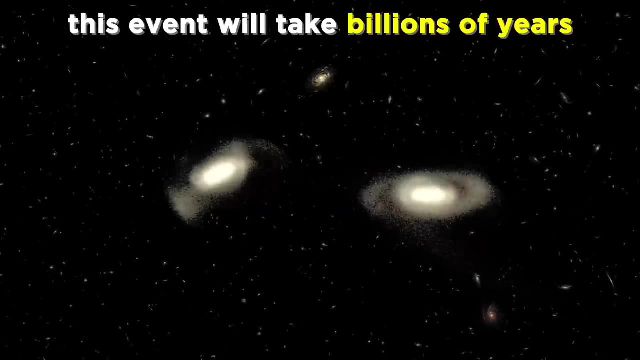 around four billion years from now. Simulations show that this will be an incredible event that will take several billion years to play out to completion. Many stars will be ejected, but the end result will likely be a very small number of stars. The Milky Way is a very large galaxy and it's a very small galaxy. 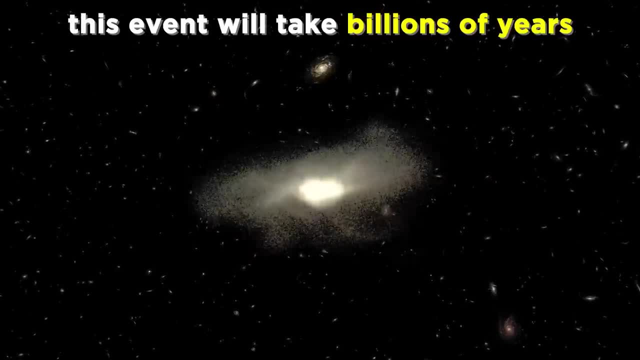 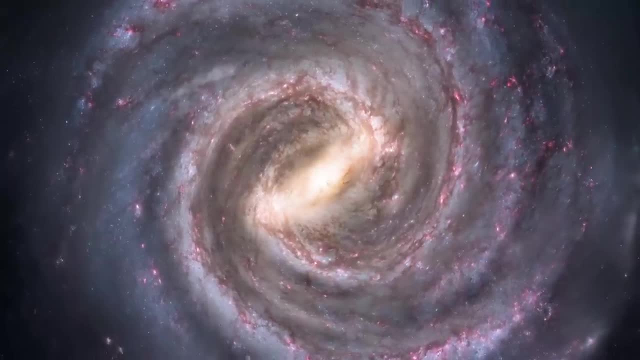 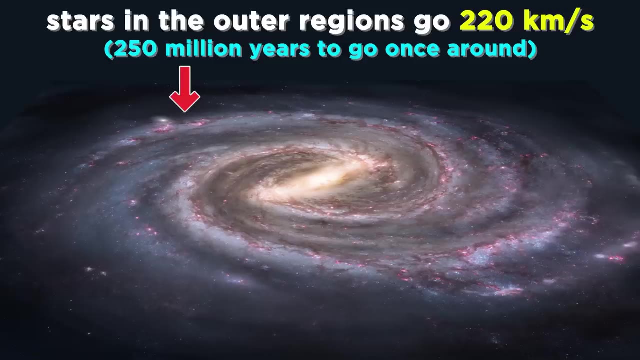 It's a very small galaxy. It will likely be emerging to form a larger, more elliptical galaxy that has been dubbed Milkdromeda. So what do we know about the formation of the Milky Way? Well, its rotation provides some information. 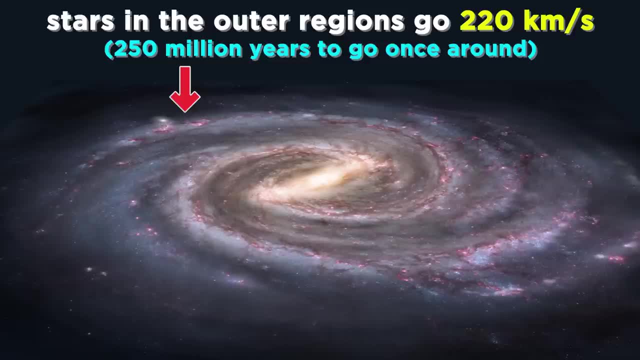 Stars outside of the bulge move around galactic center with a speed of around 220 kilometers per second. That's astonishingly fast by earthly standards, but even so it takes stars in the outer areas of a galaxy about 250 million years to go once around. 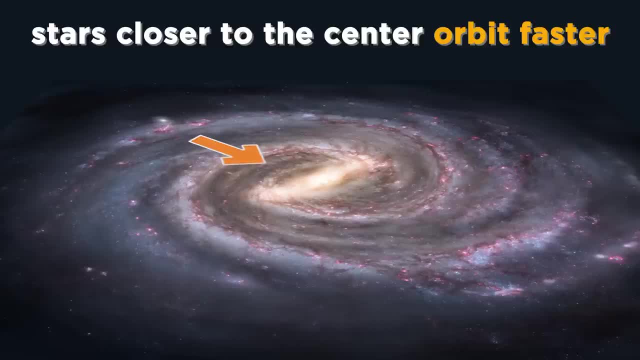 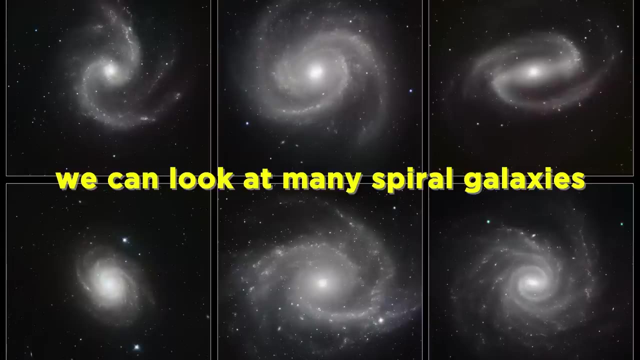 The closer stars are to the center, the less time they take to orbit, just like planets, around their sun. In fact, this is the phenomenon that is largely responsible for the formation of the spiral arms in the first place. This is all typical among spiral galaxies, as we can observe by looking at other galaxies. 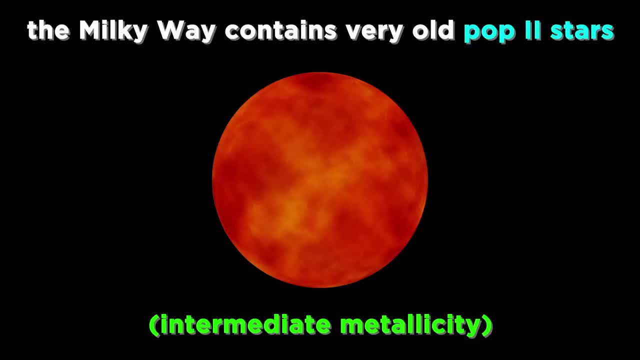 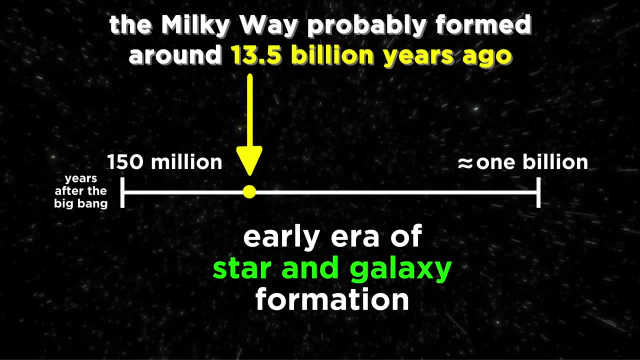 in our vicinity. The oldest stars we can see in the Milky Way are very old. population: two stars. In fact the oldest stars we can see in the Milky Way are very old. population: two stars, stars. so we believe the formation of the Milky Way dates back to that early era of